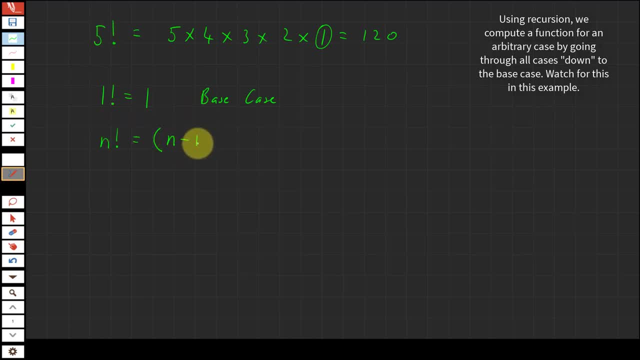 from that n or 5, we took away 1 there and that becomes our new factorial, But then we times it by 2.. Now n So if you take a look up here and take the 5, put the 5 there. 5 take 1 is 4.. 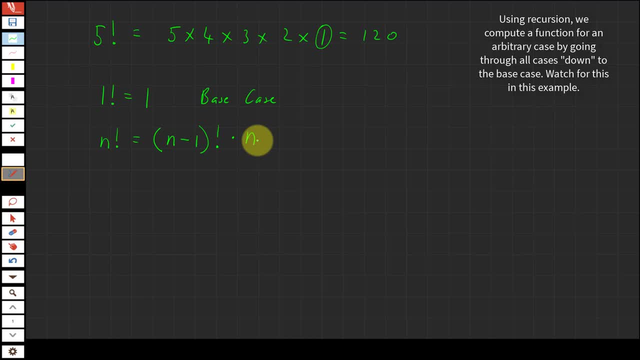 So that's 4 factorial times 4.. So 4 factorial. so in our case above, if we had 5 factorial, that it would equal 5. take 1 factorial, So 4 factorial times 5, which is equal to 4 factorial times 5.. 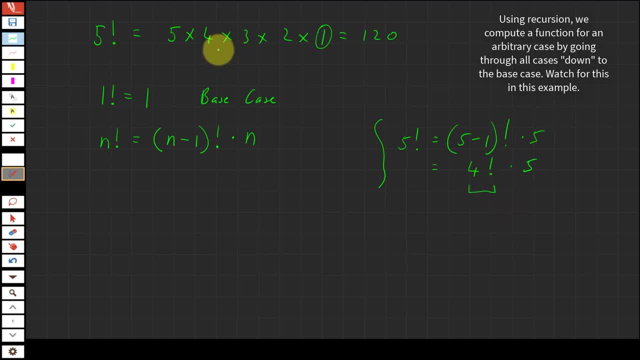 Notice that 4 factorial is actually this section here And the 5 is that part there. So this line here has given us the a breakdown of that 5 factorial, But not a complete factorial. But if we keep using this recursion step here, we will get down to the, the full breakdown. 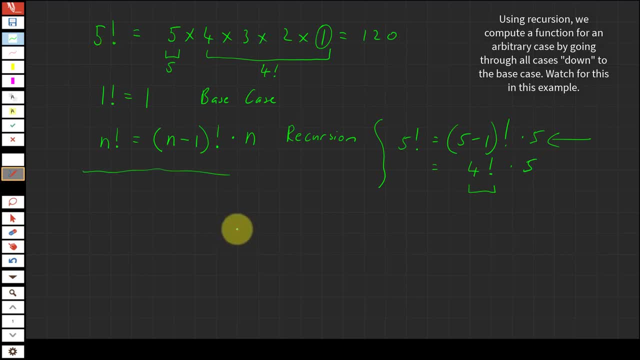 of 5 factorial or any number we choose. Okay, so let's apply this rule here to the 5 factorial and get the full breakdown: 5 times 4 times 3 times 2 times 1.. So, as we just mentioned, we start with the 5.. 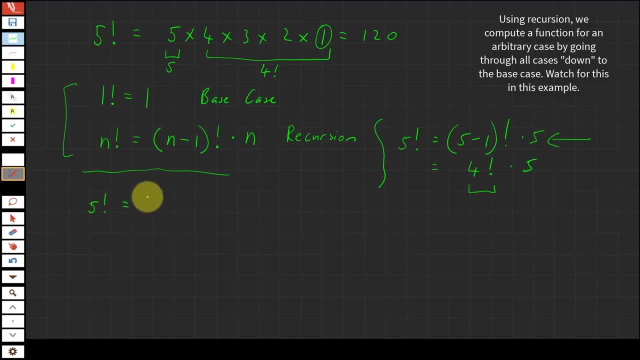 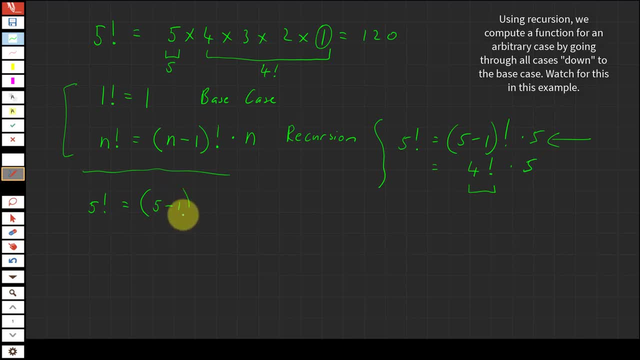 And then we get down to the 5 factorial on the left. That equals 5. take away 1 factorial times 5. Which is equal to 4 factorial times 5.. We now do the same operation, this operation, this recursion rule here to the 4 factorial. 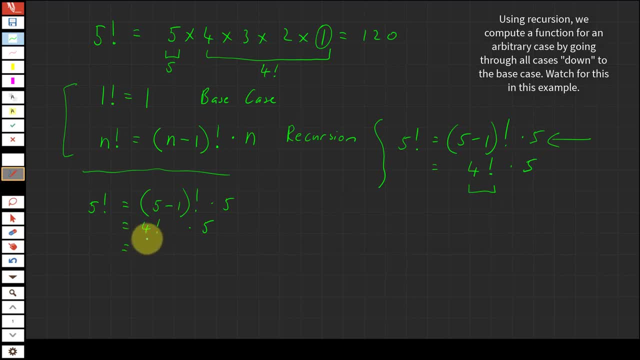 So we do that same operation: 4 factorial times 2 times 1.. 65.. four take one factorial times four. that's our recursion operation, but we still need to add that five in there. so times five, which is equal to three factorial times four times five, you can see how we're sort of starting to expand. 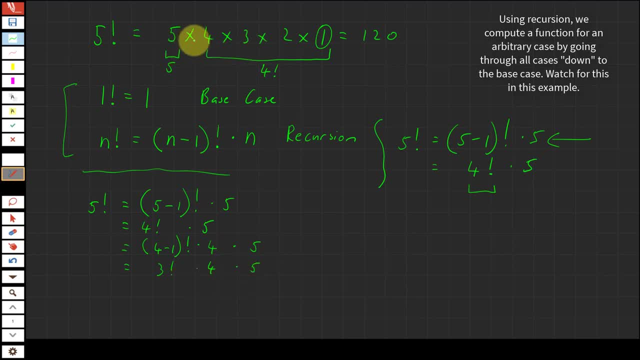 out with what we have up here. we do this same recursion rule again on the three factorial. so that is equal to three. take one factorial times three, three- we still have the four there and we still have the five there. so this is equal to two factorial times three times four times five. 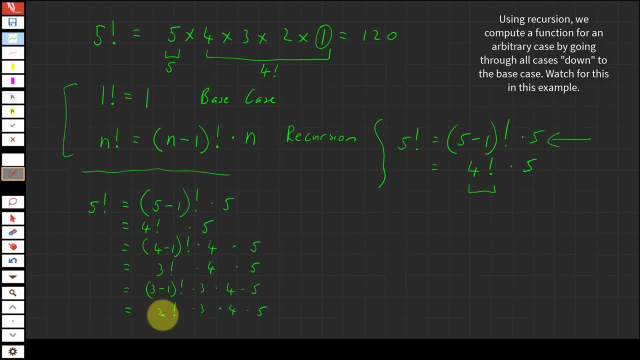 okay, we do the recursion rule again on that. two factorial, so that is equal to two. take one factorial times two times three times four times five and we'll just go up here, so that is equal to one factorial times two times three times five, five, six, seven. 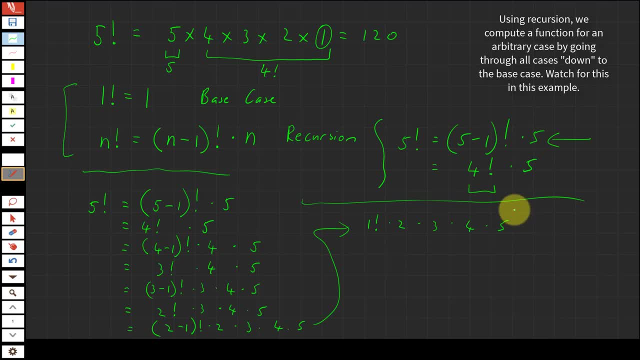 eight times four times five. but we know for now base case that one factorial is equal to one. so now we can terminate here and write: um, this is equal to one times two times three times four times five. and there we have our answer. so, um, it's just written in the opposite order here. 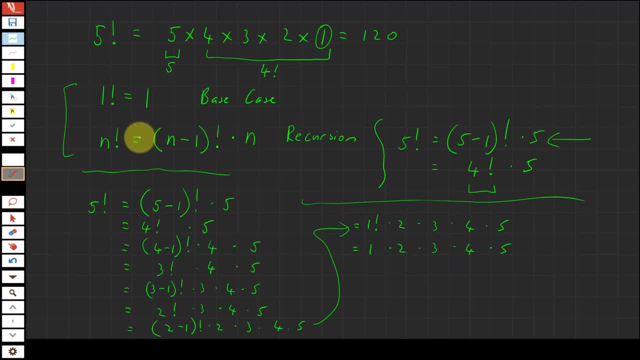 uh, because our rule is written. if we had the n on the front there we would have the same order as here: five times four times three times, two times one. but we've just written it, written it in the opposite order: um one times, two times three times four times five. so that is the principle of 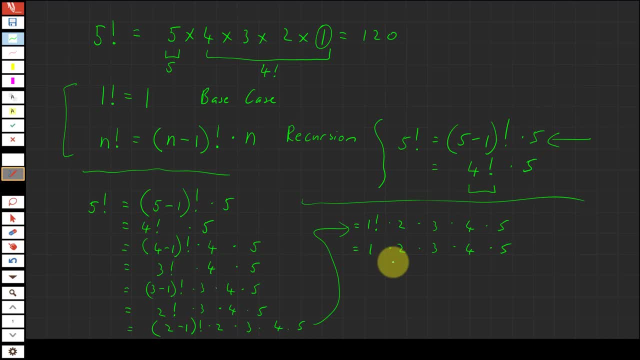 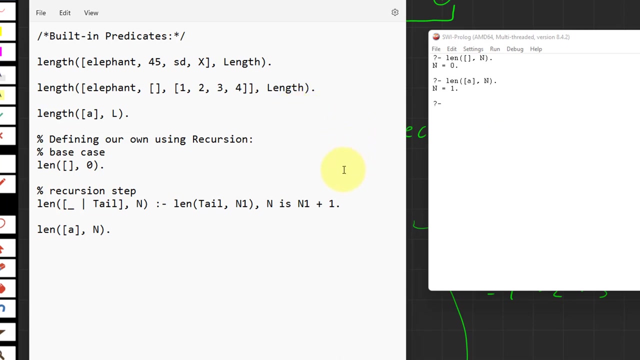 recursion and the same principle is used in prologue. to carry out recursion, we need a base case and we need the recursion rule. okay, so now let's take a look at prologue and using recursion in prologue itself and how the recursion in prologue is. 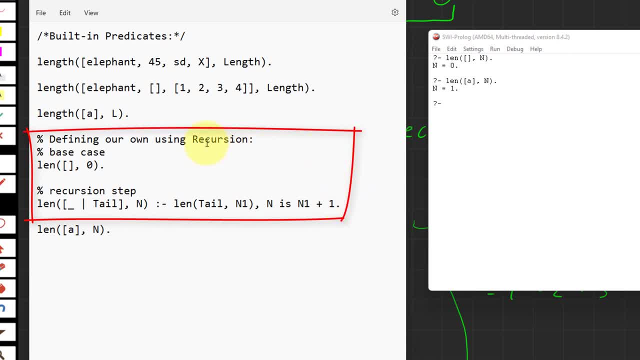 the same as recursion in mathematics. so here we've got built-in predicates, length, which are built into the prologue language, which calculate the number of elements in a list that we supply. but we can also define a recursion operation to carry out the to return the length of the list. 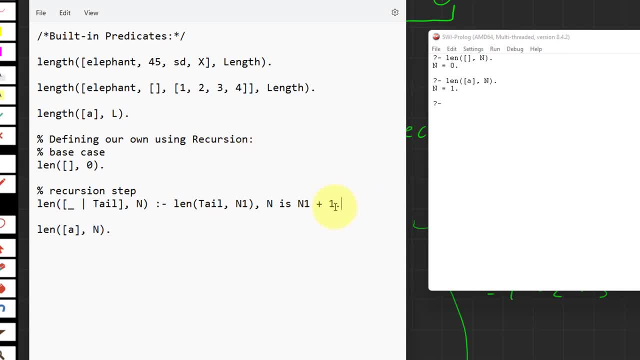 or the number of elements in the list. so here we have our recursion program here. notice, just like we did in in mathematics, we had a base case and then we had a second step called the recursion step. you can see in the recursion step, uh, we have the, the, the len function on the left and the fui function on the right of 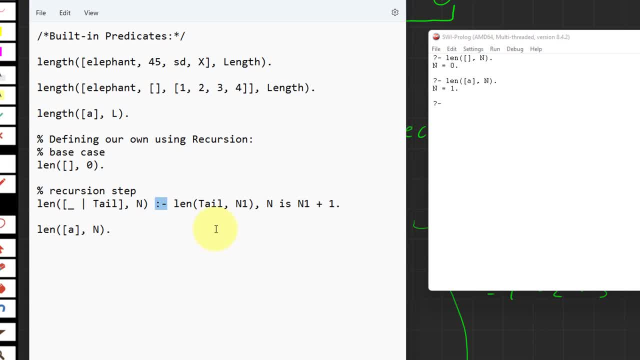 the neck operator there or the if operator there. we also have the predicate is here, remember is predicate- takes the actual left-hand side and right-hand side argument. so in this particular case it describes the value of n1, adds one and returns that particular value. on which if in prue? before, but if you have to solve this, we will cover below in those sections further next week. so things we did here inside the blues and then we using this particular case um very other way. the algorithm left hand side, which was seen in this particular case now is how that button does the. 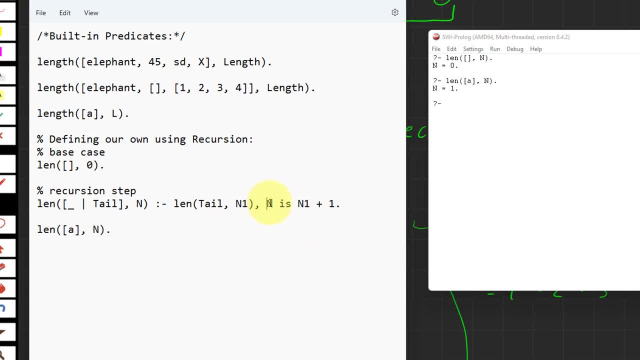 that that summation to n. so if we run this program in prologue for a empty list, we simply get 0, and if we run this program for a single element list with one element there, we get a value of 1. notice on on the on the left of the next. 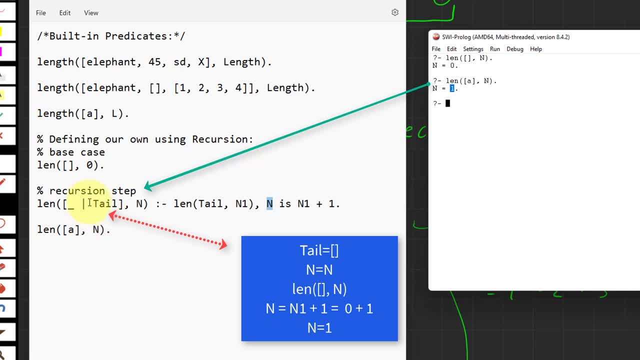 symbol or the head of this rule. we have the vertical bar here separating the head from the tail of the list. so in this particular call to the recursion program that we we supplied here, you can see there is one element to the head but there are zero elements to the head, and there are zero elements to the head and